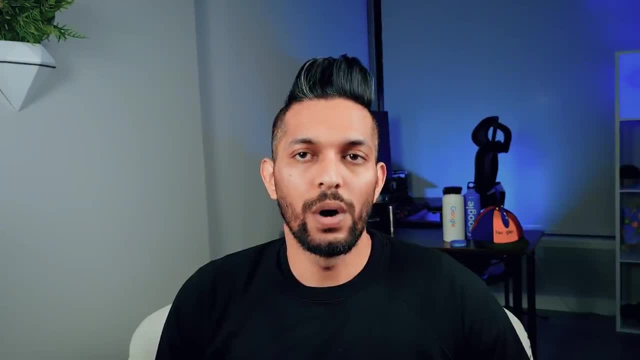 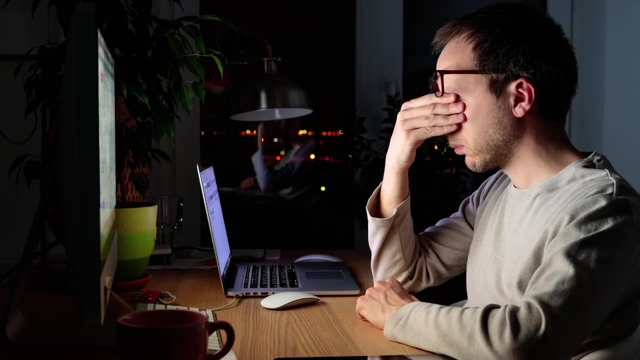 I want to share my journey with you. I'm doing it for two reasons: 1. If you're just starting out and you're completely confused about what exactly to learn, like I was, this will answer some of those questions. 2. If you're feeling demotivated because people keep telling you that you cannot become a software. 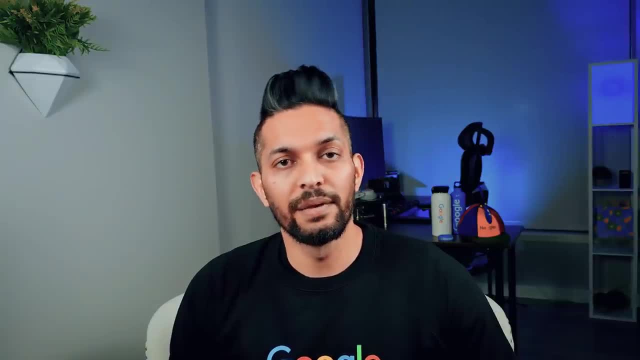 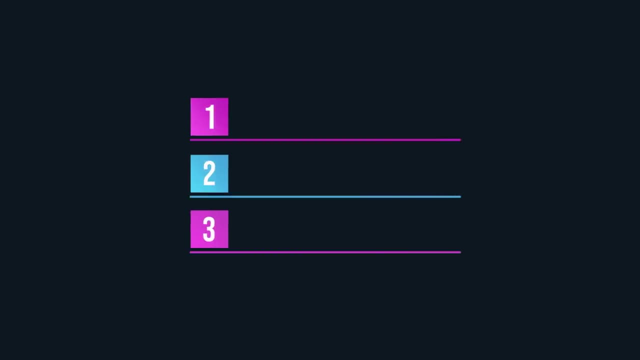 engineer without a CS degree. I want to let you know that there are ordinary people like me who have done it. You can do it too. Before we begin, there are three things that are essential for breaking into software engineering as a self-taught programmer. 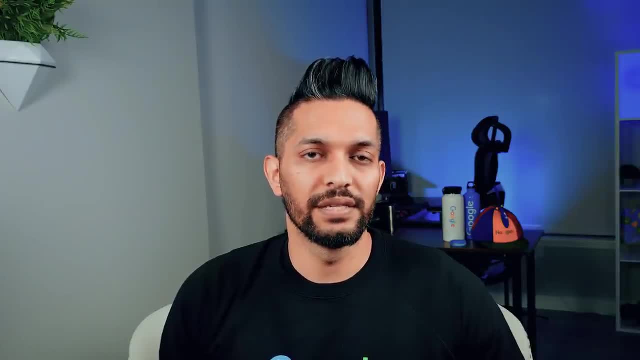 I'll share these three things as I walk through the steps I took to become a software engineer. When I first started out, I did not know that learning programming is going to be an intricate maze of choices. The very first choice I had to make was which programming language to learn. 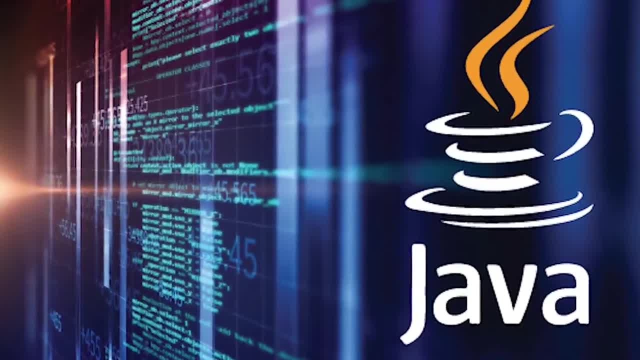 I had the option to do it the old-school way, by learning Java or C++. Another popular option was to use Python, which is much easier to learn. I had the option to use Python, which is much easier to learn. I had the option to use Python, which is much easier to learn. I had the option to use Python. 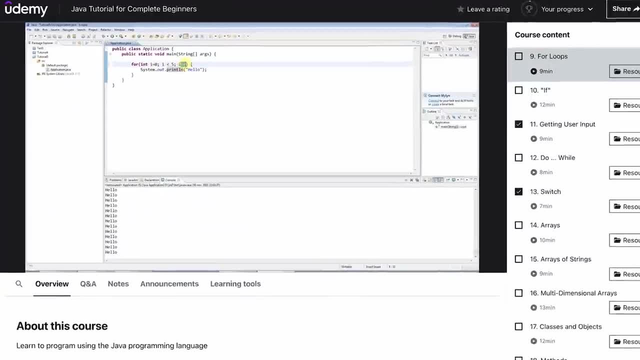 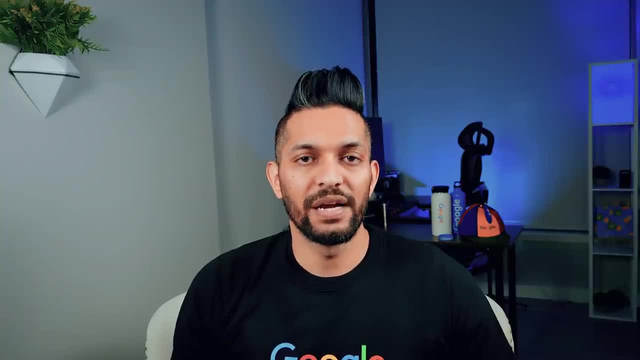 which is much easier to learn. I ended up choosing Java for two reasons. One, online courses that I found to learn Java were much more in-depth than Python courses. Two, Java is statically typed language, whereas Python is dynamically typed. What this meant in practice was that, for a beginner, Python is harder to debug than Java. 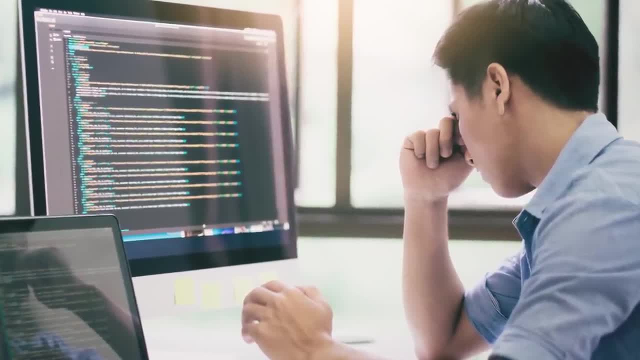 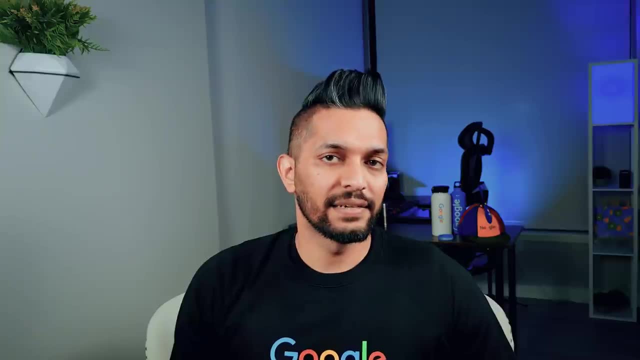 As a new programmer. we are all thrown off by that error message that pops up when we run a program, so I gravitated towards Java. Another reason why I chose Java was because I wanted to get into Android development. At the time, I thought it would give me an easy side project to put on my 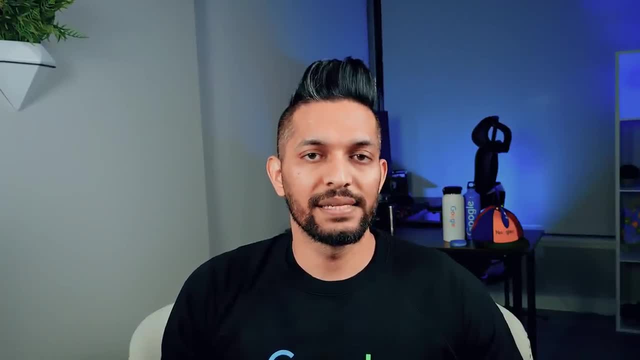 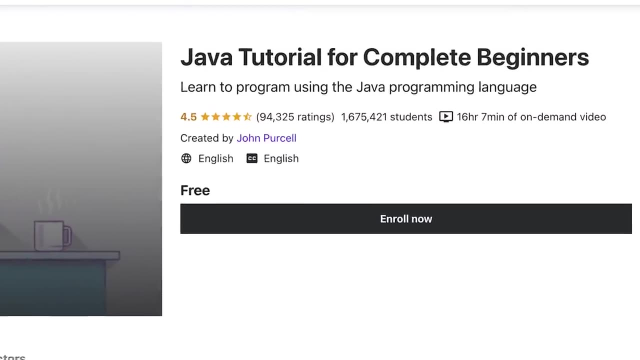 resume. As it turned out, it was a grave miscalculation on my part, as I didn't understand how complex programming can be at that time. To learn Java, I found a free course on Udemy. The course is called Java for Complete Beginners by John Purcell. This course taught the basics of 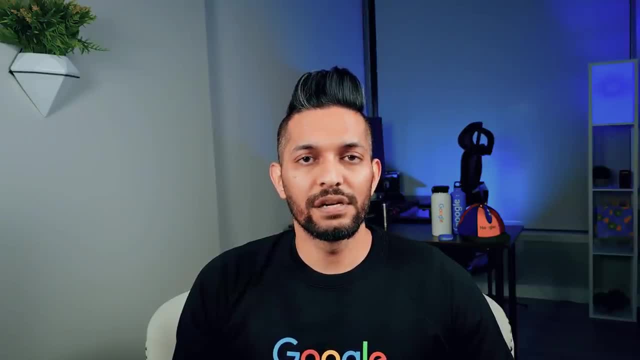 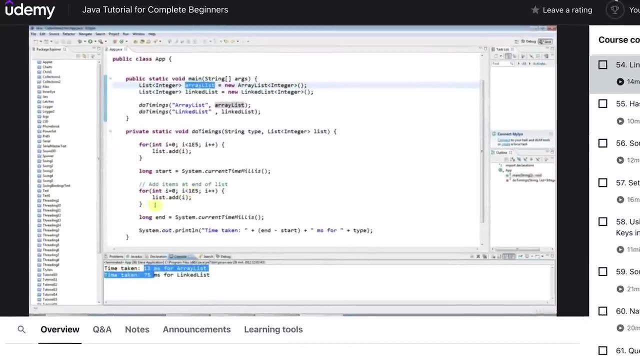 programming, like how to define variables, how to write FL statements and loops, etc. I also learned about object-oriented programming through this course. This course provided an introduction to data structures like hash maps, linked lists, queues, etc. Once I learned Java, I started working on my Android app. 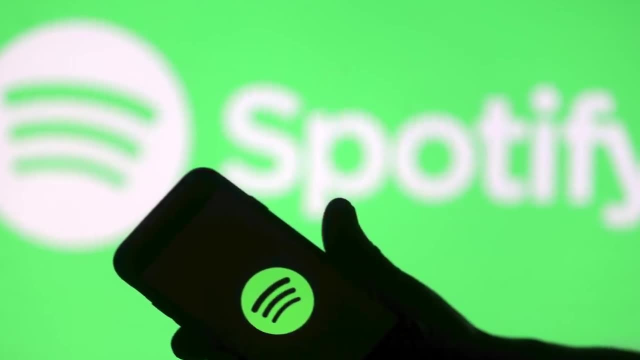 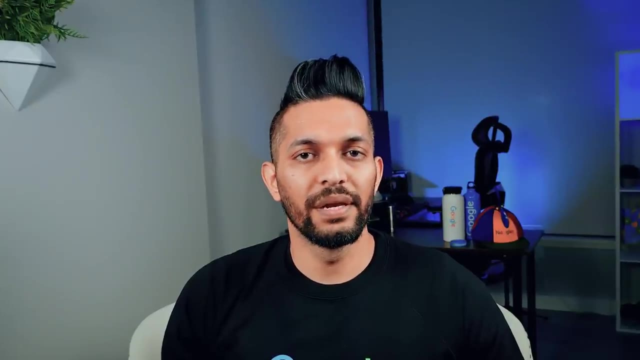 I decided to make an alarm clock that can wake you up to your favorite music on Spotify. To do this, I learned Android development using this course from Udacity. After completing the course, I was very confident about my ability to build this app. I guess I didn't know about. 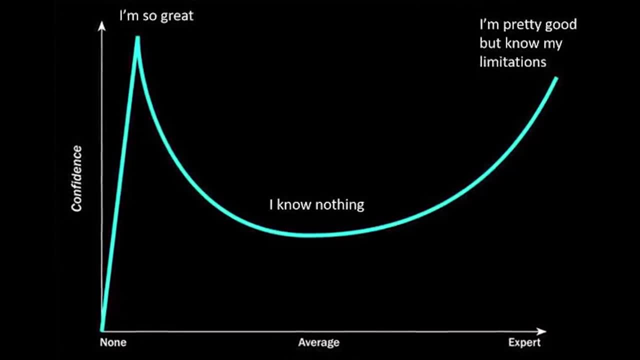 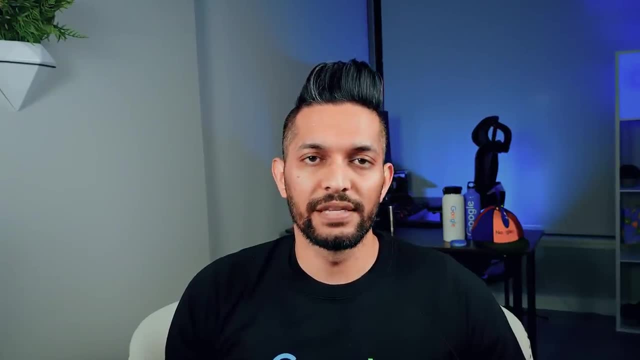 the Dunning-Kruger effect at the time. Within a couple of weeks I hit the bottom of the Dunning-Kruger curve and ran to my programmer friends for reassurance. This is where I learned the first essential thing. you'll need to break into software engineering Whenever you get out. 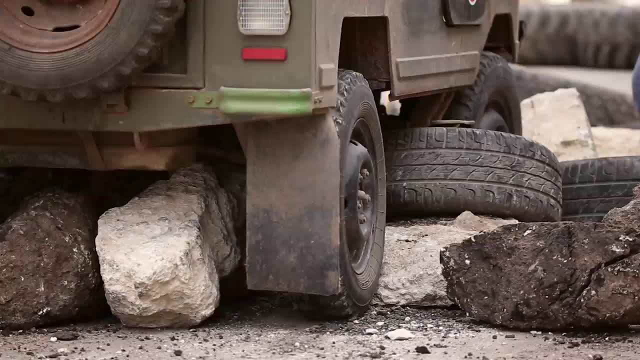 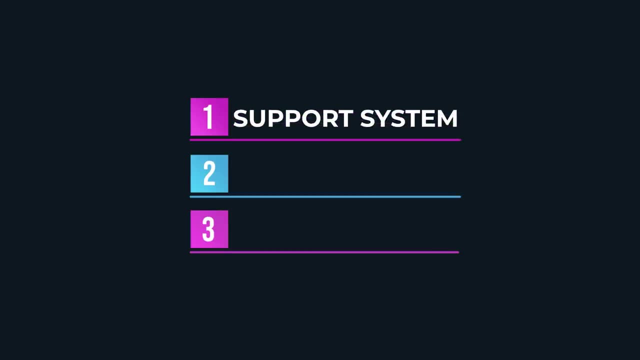 of your comfort zone and venture into a new field by yourself, you'll always face roadblocks. In the end, you'll need friends or some form of support system that will cheer for you no matter what. My friends reassured me that I was doing great and also helped me debug the issues with my app. 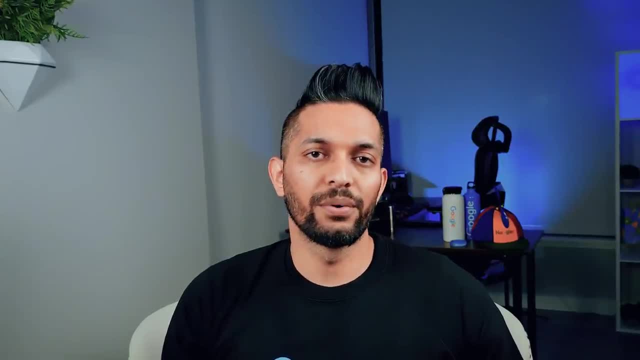 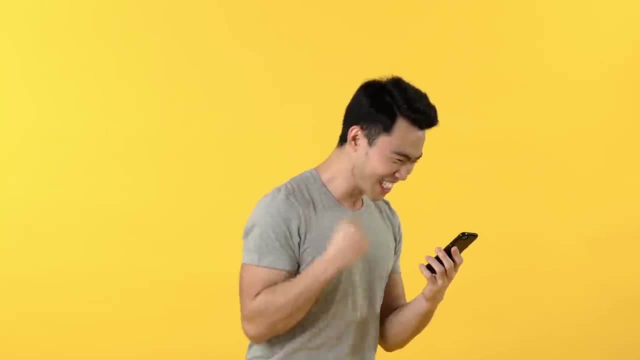 Some of them commended my coding abilities, which now, when I look back at my code, was very generous of them. In the end, I was able to finish a working app. It was not perfect, but it worked, and that gave me a lot of confidence. 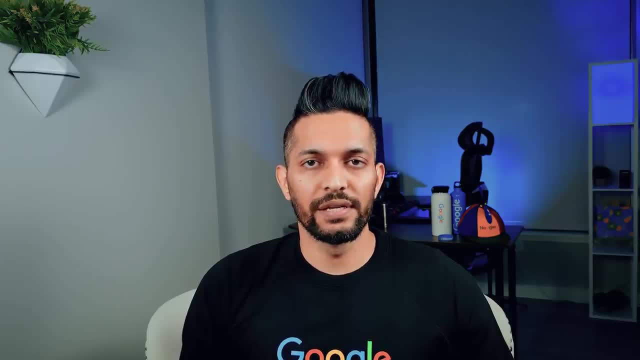 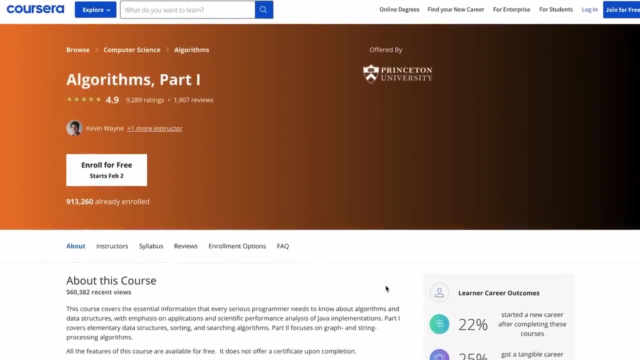 Knowing programming and having side projects is not enough to become a software engineer. You need to have a solid understanding of data structures and algorithms. to get into big tech companies To learn about data structures and algorithms, I did a free course from Coursera. 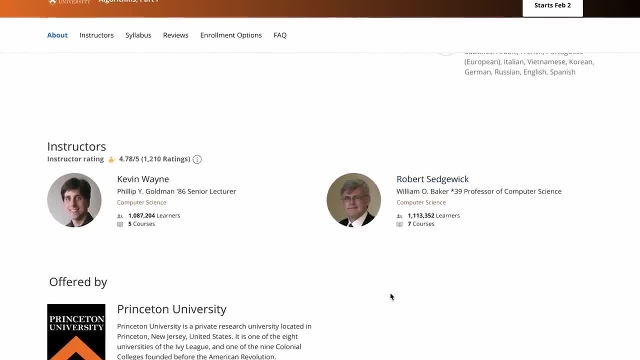 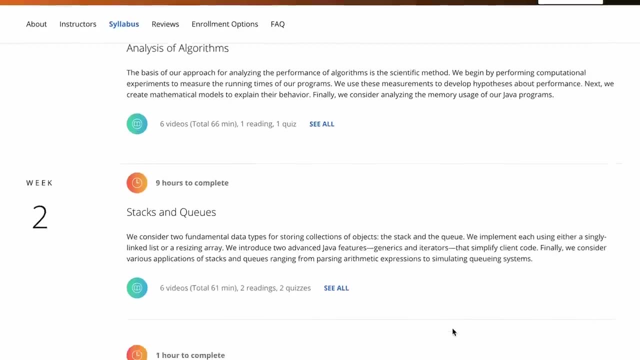 The course was taught by Professor Sedgwick from Princeton University. This course taught me simple algorithms for sorting into complex algorithms like unifying and dynamic programming. This course also introduced me to Big O notation, which is a closing question for most coding interviews. However, the best thing about this course was that it explained me the internals. 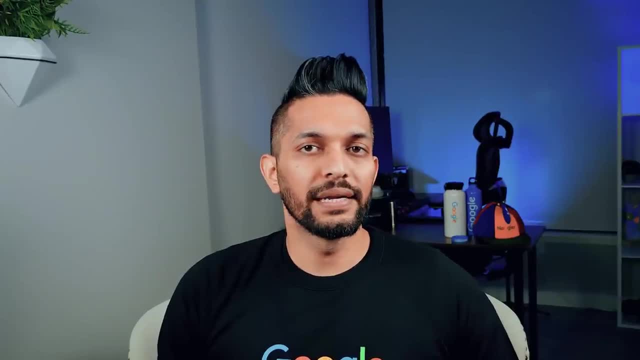 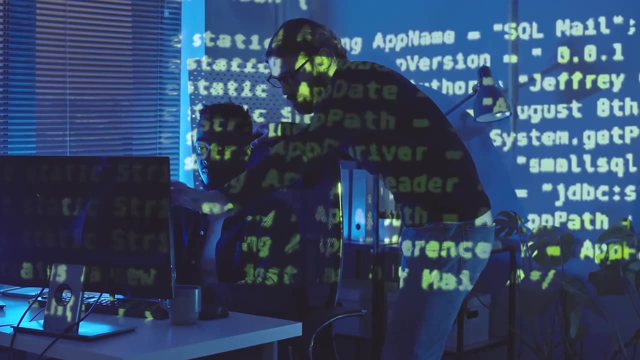 of many data structures. For example, many of us know what an array, list or list is, but do you know what happens to the memory allocation when you add a new element to the list? To this day, I come across engineers who don't know the fundamentals that are taught in this course. 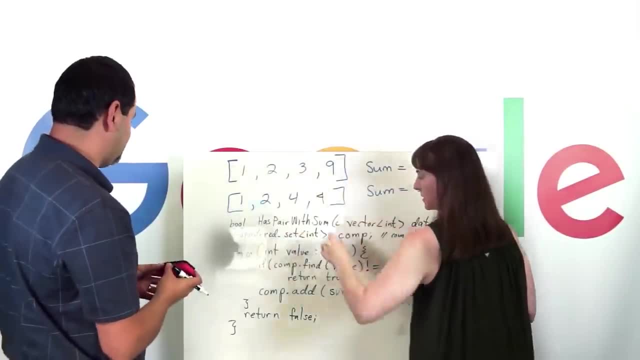 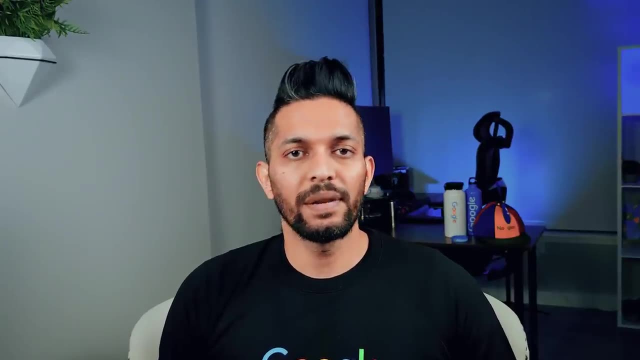 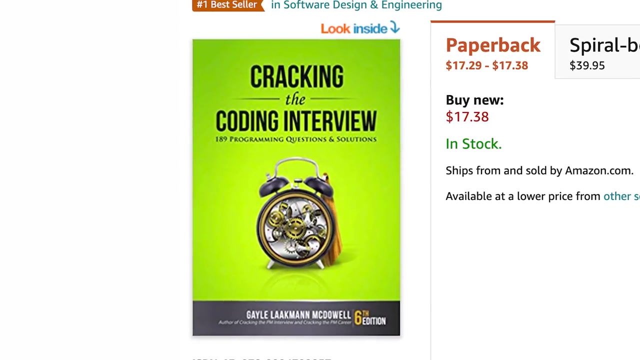 so I highly recommend this course. Knowing data structures and algorithms is one thing, but cracking the coding interviews is a whole new ball game. I had implemented many popular algorithms by myself, but applying all these algorithms to a new question under the time pressure of an interview was going to be very difficult To sharpen my interview skills. 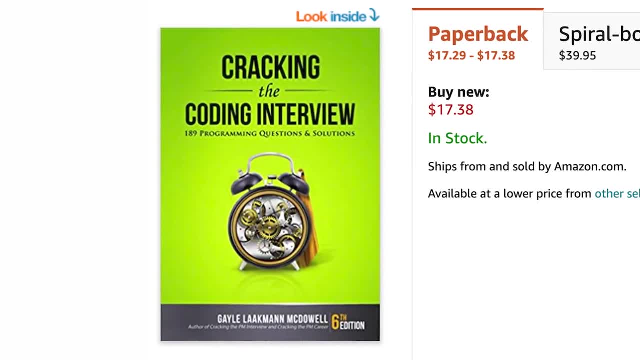 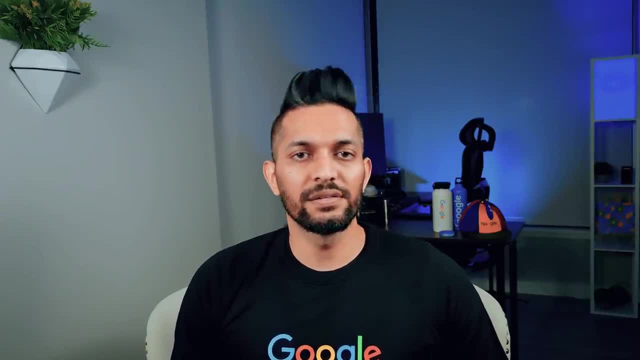 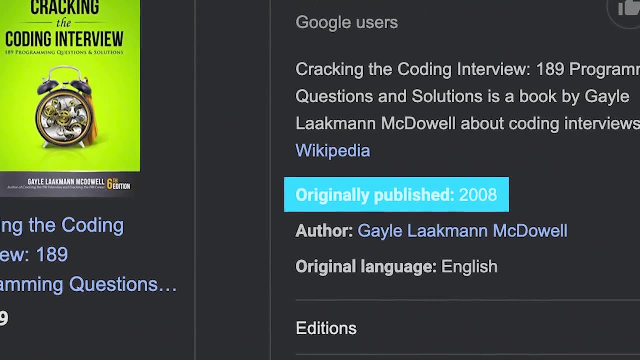 I chose to practice interview questions using a very popular book called Cracking the Coding Interviews. This book covered all the theory needed for interview preparation and it also introduced me to some popular interview questions and their solutions. However, this approach had two major problems. One, this book was originally published in 2008,- and the landscape of tech. 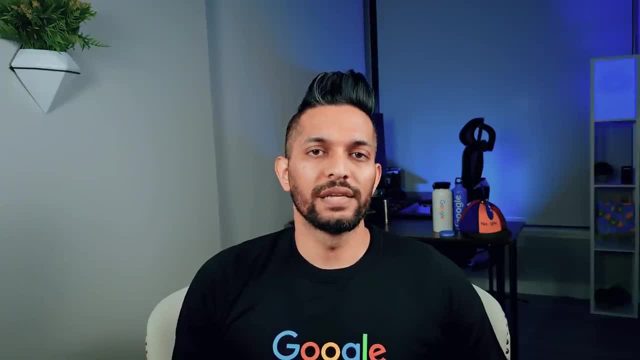 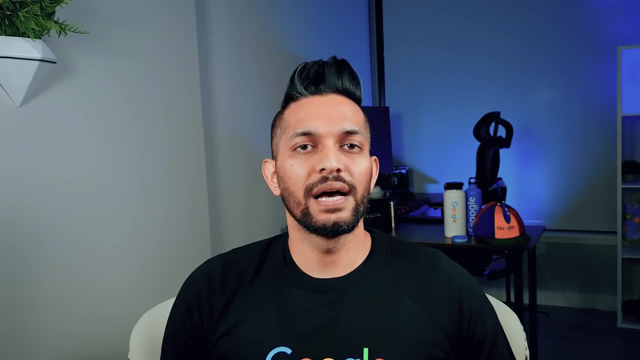 interviewing has changed a lot, since More and more people want to get into software engineering now, and thus the field is much more competitive. The questions in the book are a little outdated and don't represent those that are currently being asked in tech interviews. 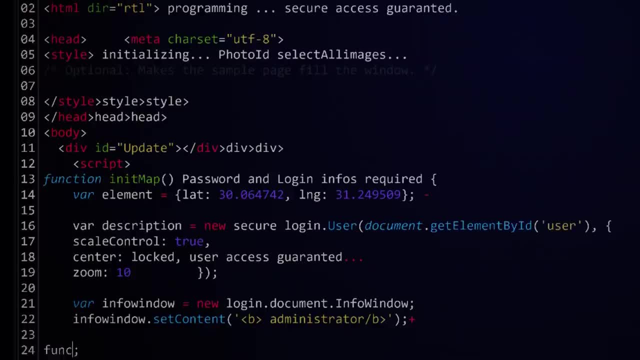 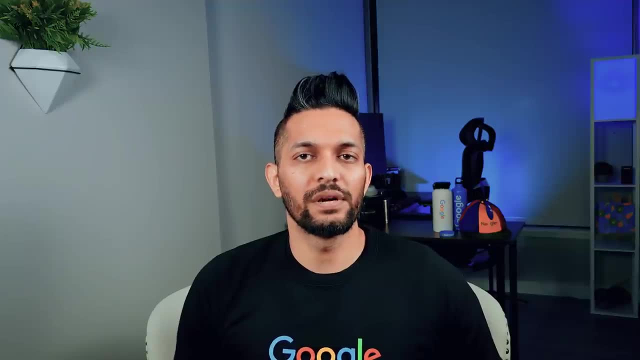 The second major problem with using the book was that there was no easy way to practice the interview questions from the book. Even if you write a solution to a question locally on an IDE, there is no way to know if your solution is robust enough to pass all the tricky test cases. 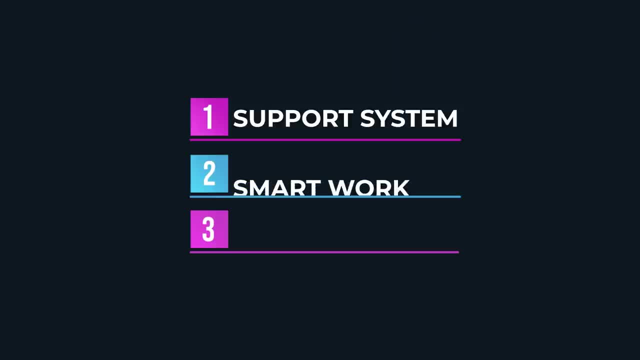 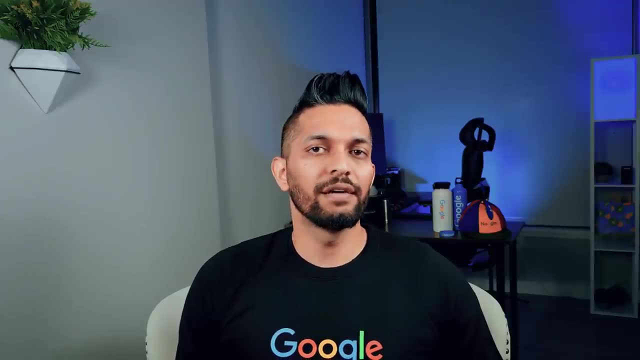 And this is where I learned the second essential thing: you'll need to become a programmer. You have to work smart, not hard. If you encounter friction using any tool to learn programming, more often than not someone has already developed a better tool: Knowing what tool to use. 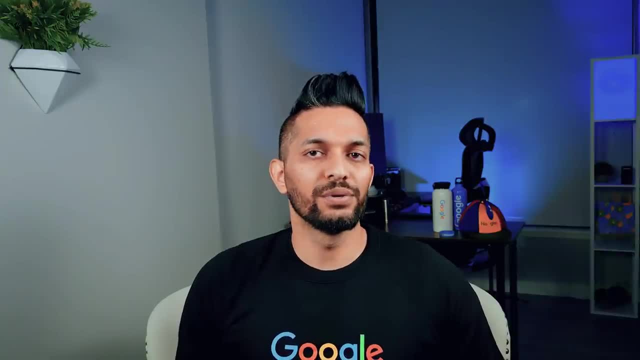 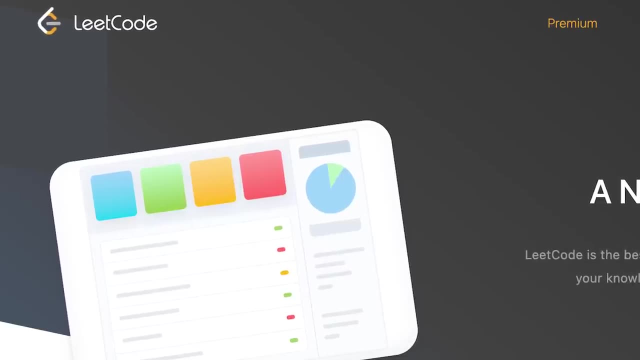 and how to use it effectively is much more fruitful than working hard using an outdated tool In the case of interview preparation. I found out about this very popular free website called LeadCode where you can practice questions for tech interviews. Questions are marked easy, medium and hard based on difficulty level If you pay for their 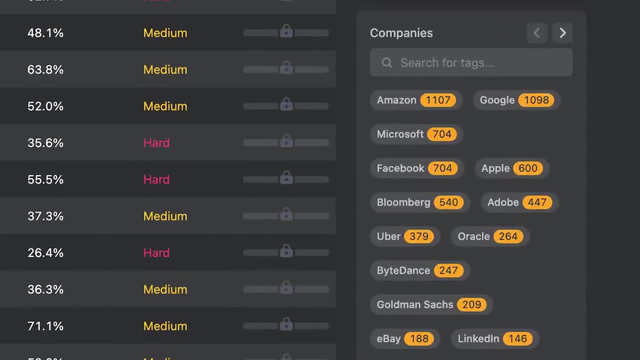 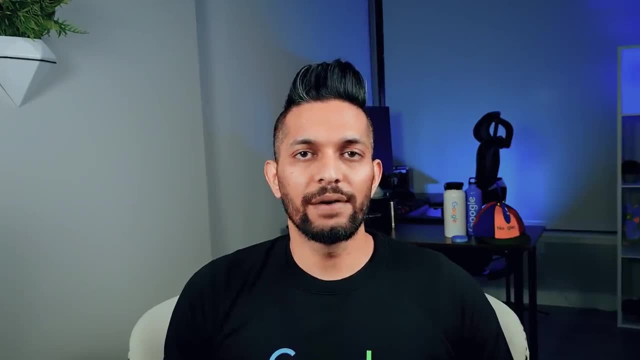 premium version you can also find out questions asked by a particular company in the past. This can help you streamline your preparation if you're targeting any particular companies. As I honed my interviewing skills, I was also looking for more projects to build my resume in. 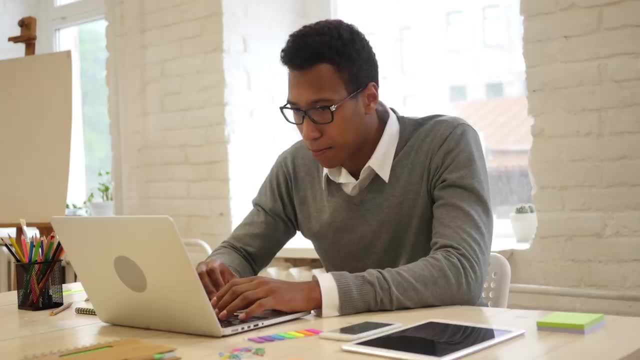 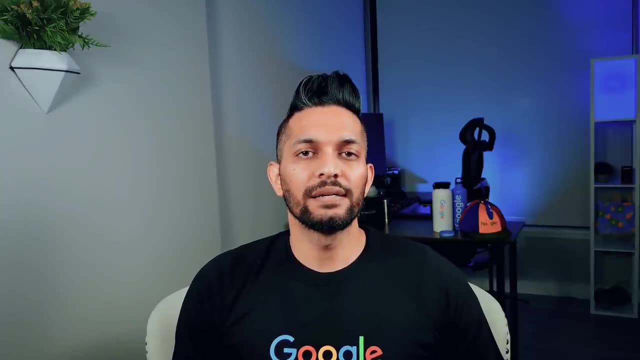 I was hearing a lot of terms like frontend and backend. Believe it or not, I did not understand those terms at the time. In order to learn about what frontend and backend exactly means, I started learning web development. I took a course on how. 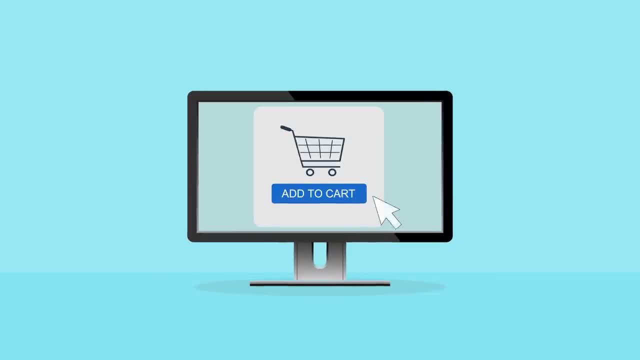 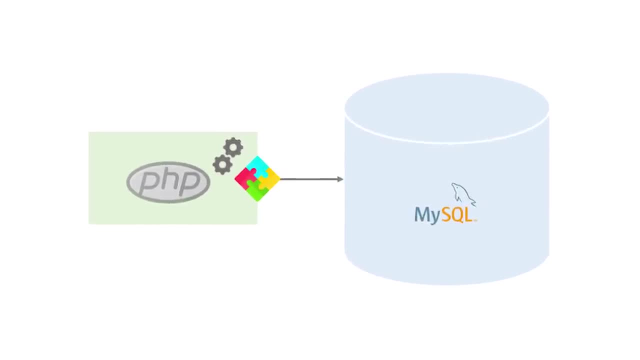 to build an e-commerce website from scratch using PHP and MySQL. In this course, I learned how to hook up a MySQL database with PHP in the backend and dynamically show this data in the frontend, Though this course provided me with a good introduction to full stack development. 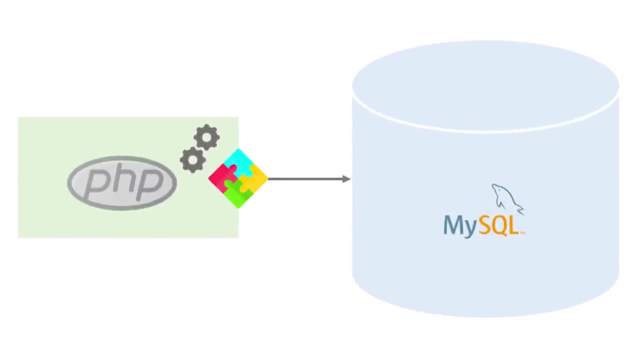 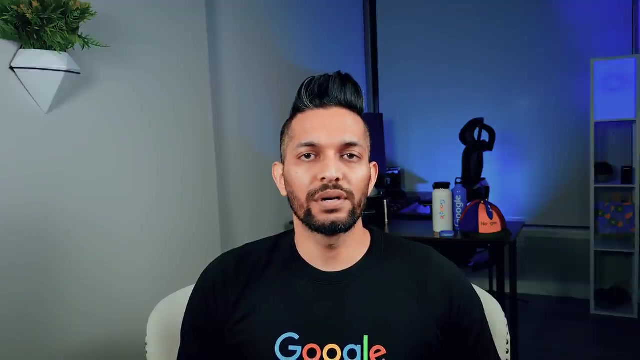 it also served as one of the many mistakes I made on my journey to become a software engineer. As I already mentioned, software engineering is an intricate maze of choices. Knowing what to work on is much more important than working hard. As it turns out, Manila PHP is not used much these days. 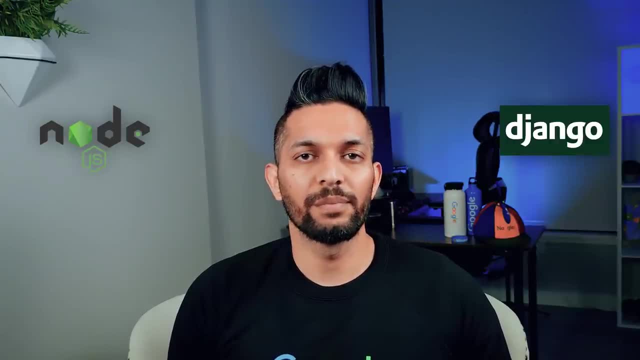 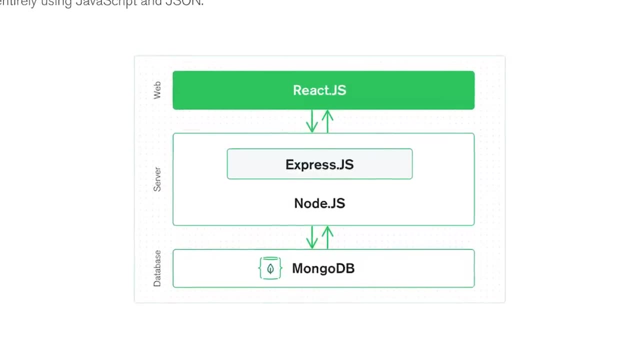 For that matter, there are frameworks like Node and Django that are not even based on PHP and are more popular. When I realized this, I quickly pivoted to learning MernStack, which includes MongoDB for Database, Express and Node for backend and React for frontend. 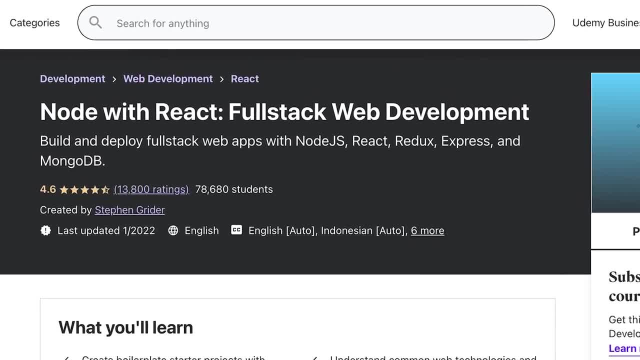 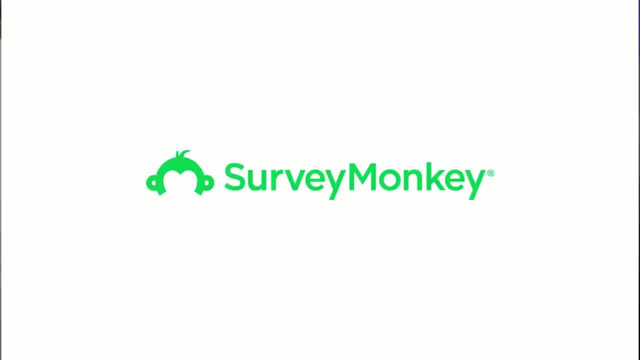 To learn MernStack. I did this course called Node with React on Udemy. By following this course, I built a website that can be used to send out survey requests in bulk through email, pretty much like SurveyMonkey does. This course served as my introduction to NoSQL databases. 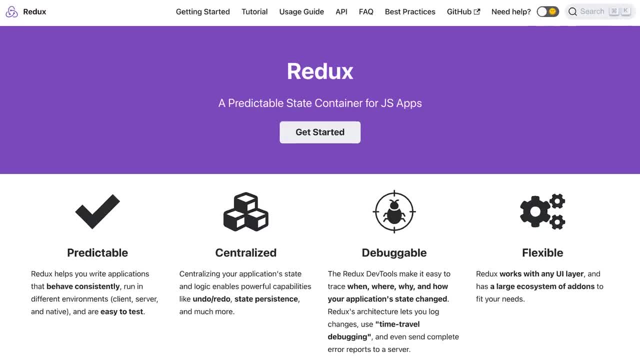 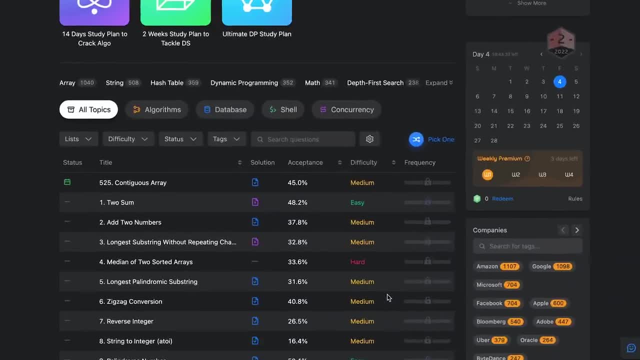 I also learned how to build single page web apps using React and how to manage the state of your web app using Redux. Along with learning web development, I was also doing two leetcode questions a day. By the time I finished my course on web dev, I had completed more than 100 questions.